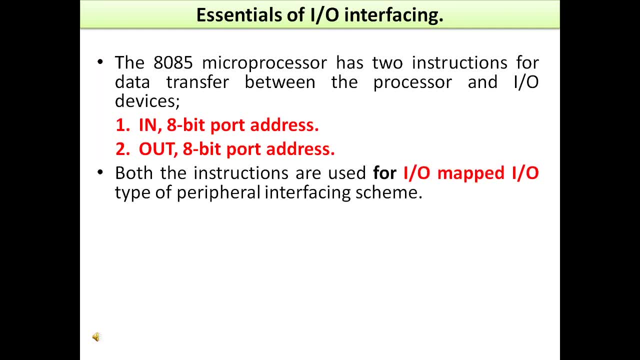 Both these instructions are used for IO mapped IO. type of peripheral interface scheme. IO mapped IO is often known as peripheral mapped IO also. Now it is a two-byte instruction and the second byte is 4B. 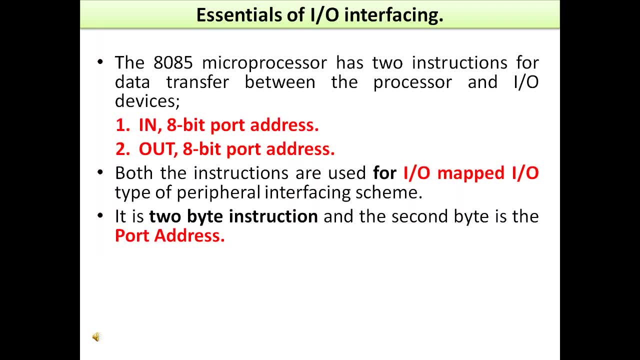 The second byte is 8-byte. If the second byte is a 8-byte then there are possible combinations 256.. So a total of 256 types of ports are possible for in and out. The second byte is 8-byte. 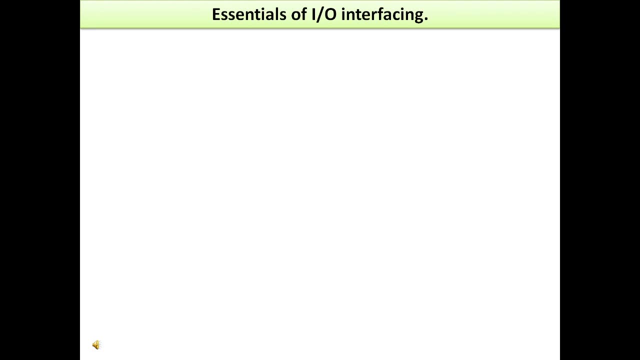 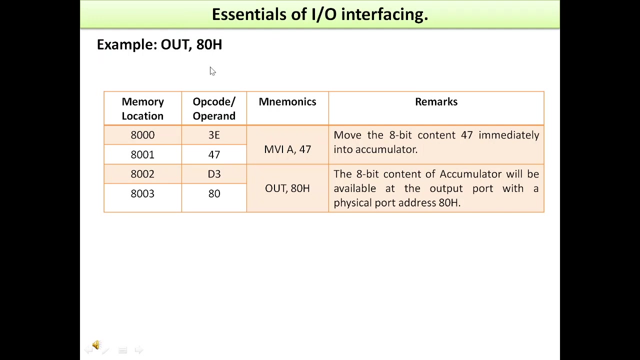 The second byte is 8-byte. Let us try to understand how the instruction works. Let us try to understand how the instruction works. Let us take an example of, Let us take an example of out instruction. now the example here is out: comma 80 hex. here the 80, 80 hex means the port address. 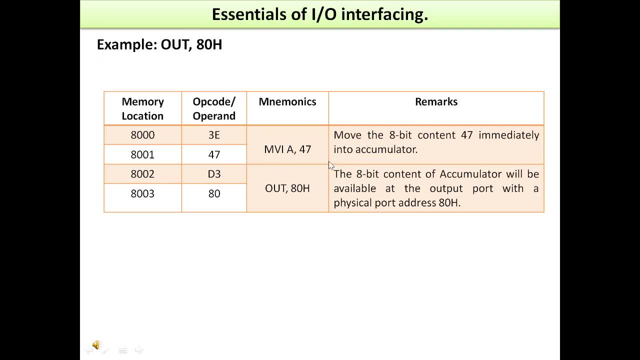 now suppose we are writing the program across the memory location 8000, 8001, 2 and 3. now in this case this first instruction means mvia 47. here it means load 47 immediately into accumulator. now, after the execution of this particular instruction, 47 will be written into accumulator. 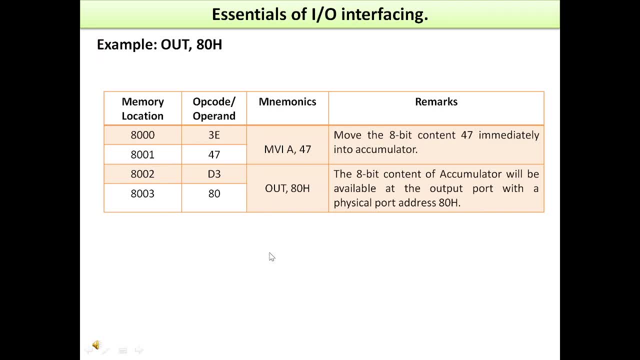 now the next instruction is out 80. now, whether we are talking about in instruction or out instruction, both this instruction are attached with accumulator. so when the microprocessor is going to execute this particular instruction, it will. it will see what is there in the accumulator. so out 80 hex means the content of accumulator. 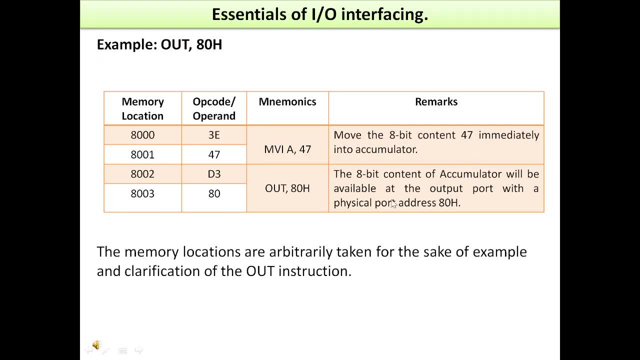 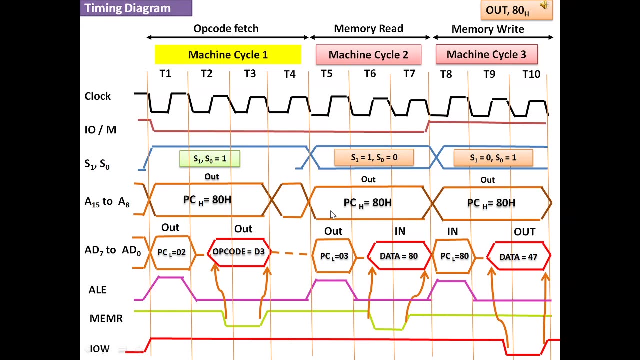 that was previously 47, will be available at the output port whose physical address is 80 hex. let us look at the timing diagram of out 80 hex now. before we try to understand the timing diagram of out 80 hex, we need to first understand that the first four t states that is the first machine. 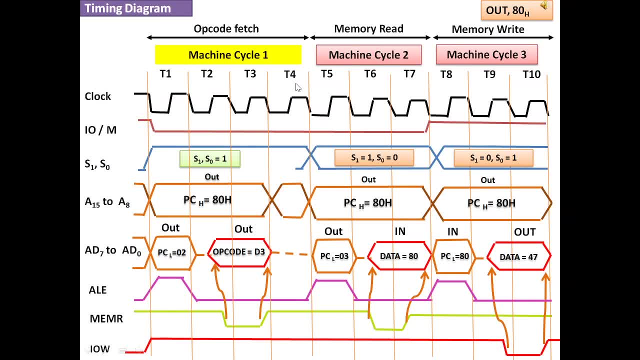 cycle is meant for fetching the operational code. the next cycle. either it will be completely dependent on the previous operational code. if the machine requires for a memory read, then there will be a second machine cycle, or if again the machine requires another machine cycle, then there may be a third machine cycle. it all depends on the operational code that was decoded. 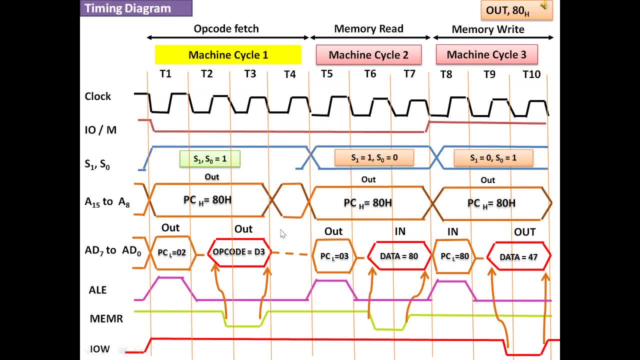 inside the machine. so let us first consider the output fetch. in this we have four t states, namely t1, t2, t3 and t4. now if we consider the out instruction, which was previously mentioned, where the out instruction was written across the location 8002 and 8003, so at corresponding to 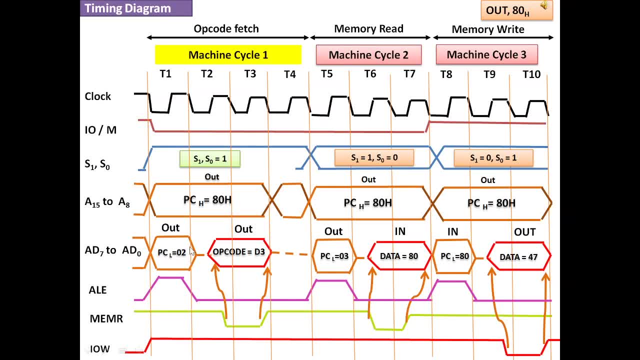 8002 the operational code of out was written. so first of all the microprocessor needs to read the operational code, or actually fetch the operational code, and then the operation of out is the operational code. decode that and only then the machine will be able to understand what sort of operation is required. now, in the first T state it is. 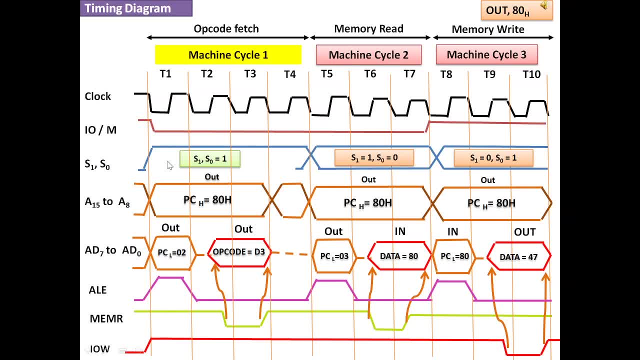 basically the addressing mode. so here you can see it is working with the memory. so IOM bar is low. now s1 and s0 are all one means it's in the FET cycle and the upper address bus is presently having 8: 0. so the upper address of from. 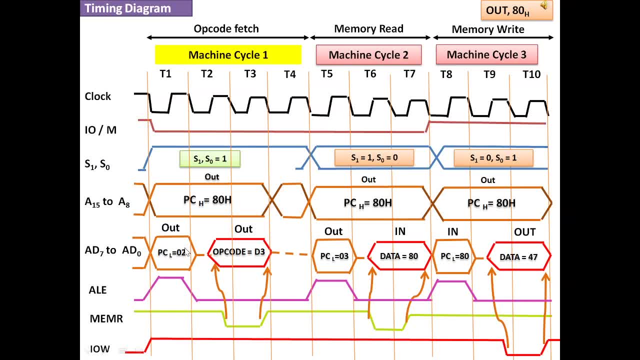 where the operational code will be fetched is in the upper address bus. the lower order address bus is having 0: 2. that means the total address is 8 0 0, 2. now in the next T state, that is 2, 3 here, T 2 and T 3, the lower order address bus. 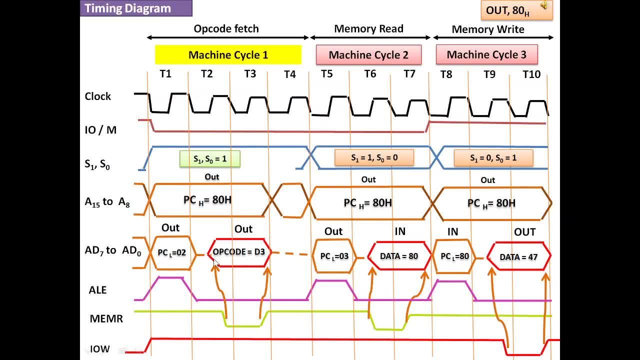 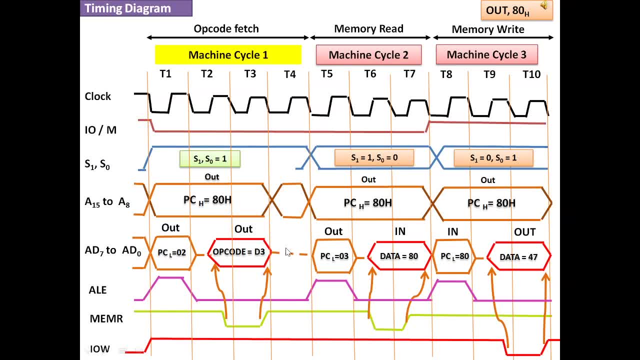 will be released and the operational code will be taken inside the microprocessor. the operational code of out is d3, and hence it has now entered the microprocessor. the machine gets ready in the T 4 state, but it is incomplete, so in order to complete the cycle it has to read the port address. 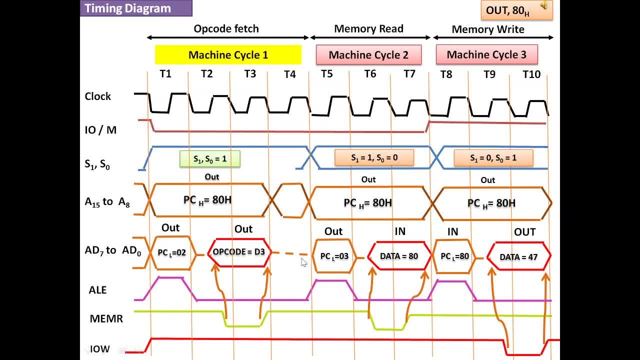 where it will be a memory read and the similar process will be on where the operational code- sorry, the operand or the data or the physical address, that is, 8, 0, is available across 8, 0, 0, 3. so again, the first t state will be meant for addressing and the last two t states, that is. 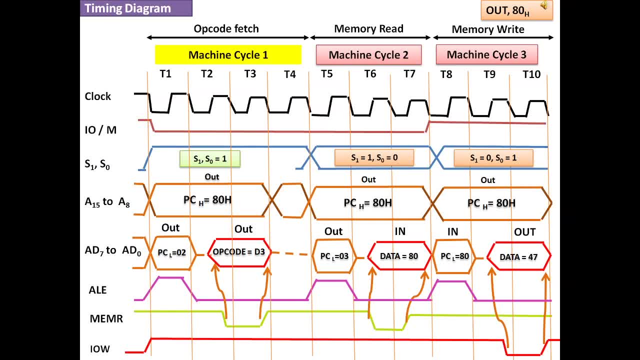 t6 and t7 of this machine cycle will read the data into the microprocessor. now the microprocessor is having the physical address inside it in the third cycle. since it's out, that means something is going to go out of the microprocessor, so it will be a io cycle. that that is why iom bar is. 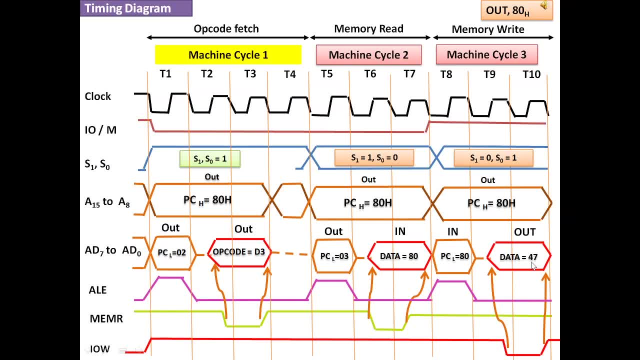 now high and it will be in a. it will be a memory write cycle. so in the first t state we can see that the higher address bus is also having the 80 physical address and the lower order address bus is also having the same physical address. so we 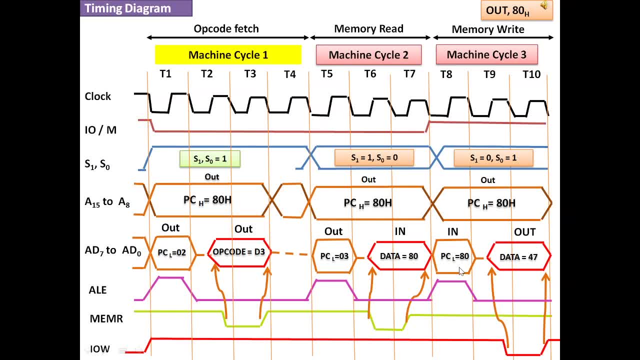 have to remember one thing: in case of 8085, for the simplicity of decoding, the manufacturers have created the microprocessor in such a manner that whenever instruction is executed, the upper address bus also carries the same physical address as well as the lower order address bus. so the system manufacturers and the board system manufacturers. 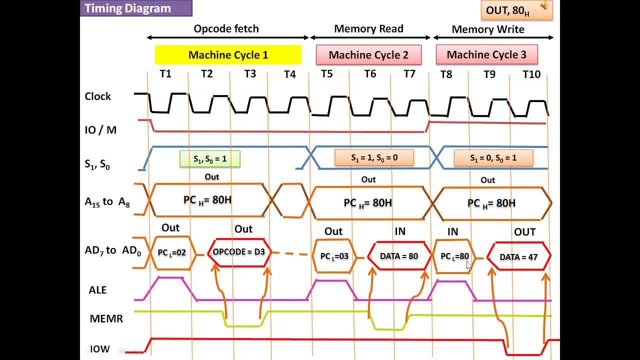 can decide whether to use this for decoding purpose or this for the decoding purpose now, since we have the physical address right now in the microprocessors program counter. now the lower order address bus is again released and the 47 that was initially inside the microprocessor is now written into the port having the physical address 80. 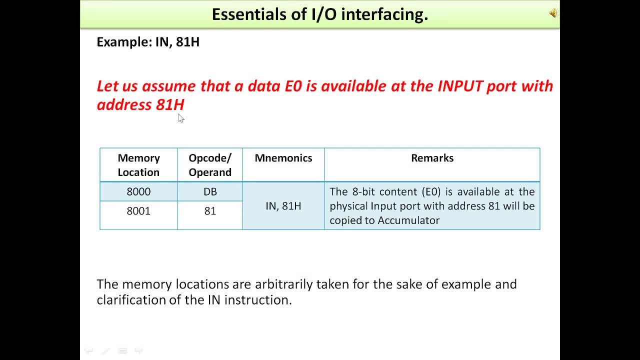 similarly, let us try and understand the in instruction. in this example we can see we have a address in, when x, here the in, is the operational code of instruction that needs to be executed and 81 is the physical address. and let us assume that it has been written across the memory location 8001. 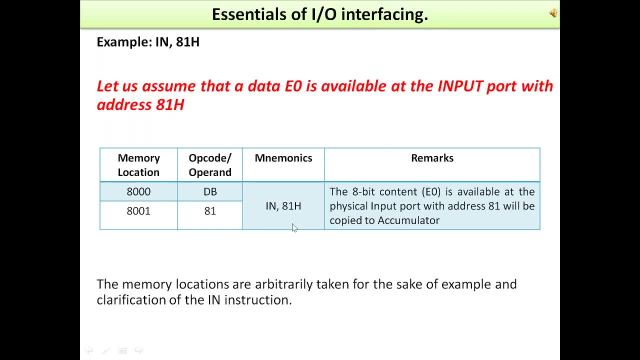 where DB is the operational code of in and 81 is the physical address. now we we have already seen that the accumulator is by default attached with these two instructions. so here anything which is available in the input port, in the input physical port, at the physical address 81, suppose it is E0. so after the execution of this, 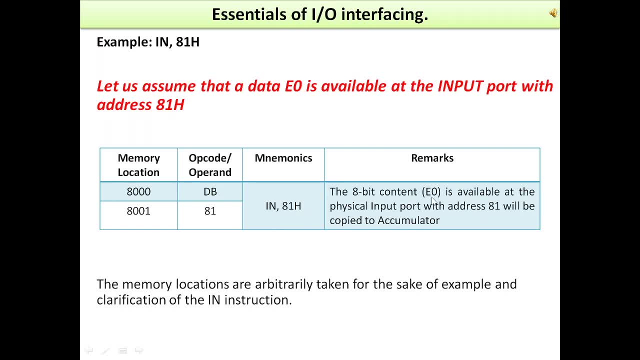 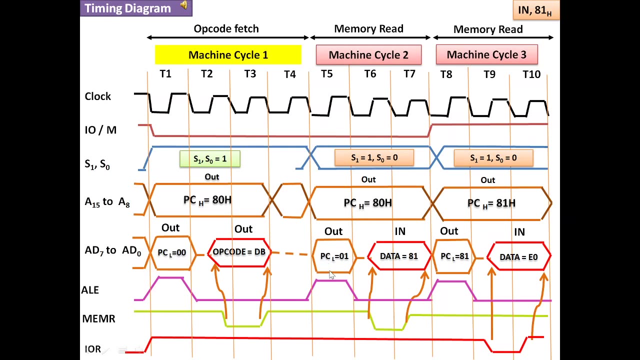 particular, instruction E0, which was available in the input port, will now be written into the accumulator. now let's again see the timing diagram. it is exactly similar to the out instruction, but only the similarity is the last machine cycle, where it is a memory read, because the the information from the outside world that is in our 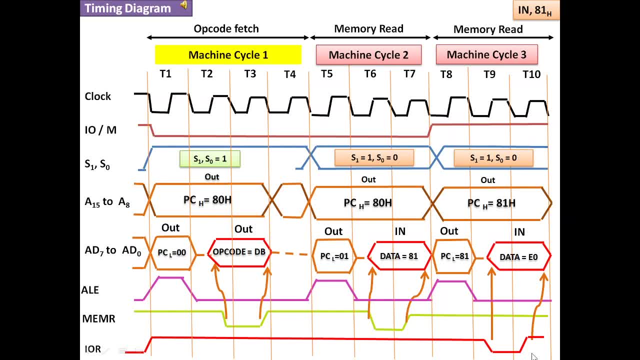 example, it is E0, which is available in the input port, is E0, which is available in the input port, is now going to get inside the microprocessor. so whenever anything is going inside the microprocessor, it is in, it is read and anything going out of 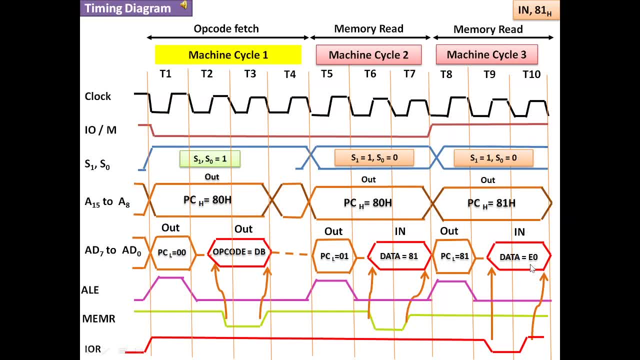 microprocessor, it's right so again, and the first machine cycle, the operational code is fetched, and and then the execution and the t4 state is partial. here everything is kept ready inside the microprocessor so that the information that is presently available at the input port will be written into accumulator. 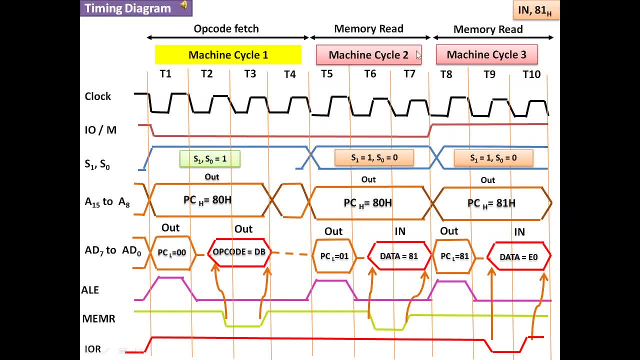 in the next, in the next machine cycle, the 81, that is the physical port address, is read by the microprocessor in the similar fashion it is read by the microprocessor as is evident from him, as is evident from this, and in the third machine cycle we can see that the accumulator content that is present in the 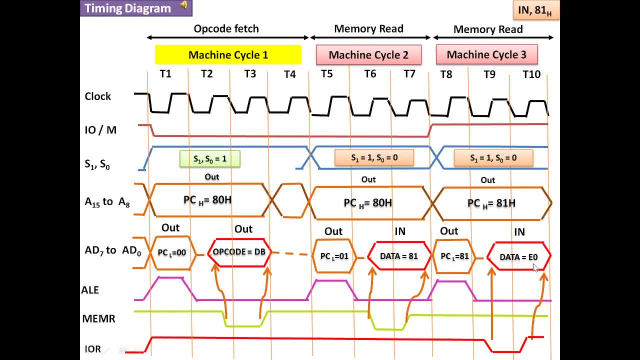 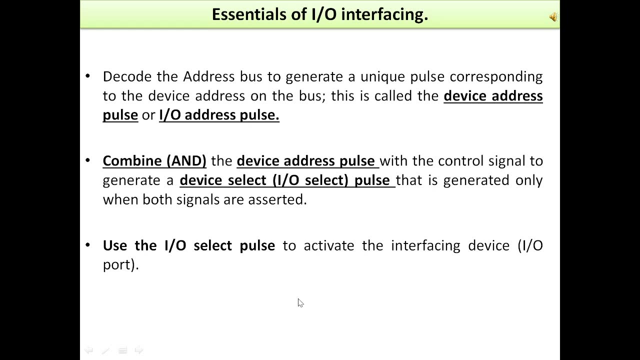 will now be filled with the available data, that is, E0, which is available at the physical port of the input port. Now let's see the procedure, how the interfacing is carried out in IOMapped, IOMethod. The first thing that we need to do is decode the address bus to: 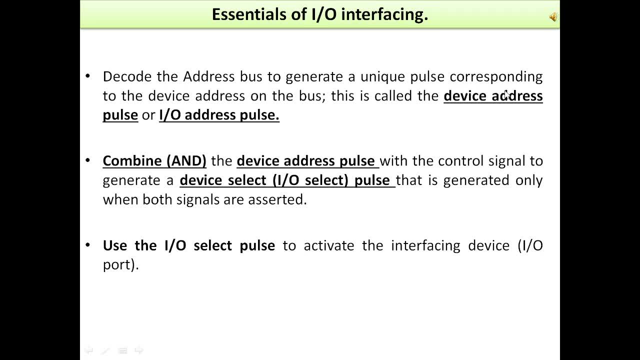 generate a unique pulse corresponding to the device address on the bus. this is called device address pulse or I-O address pulse. Now we have to combine the I-O address pulse with the deviced select pulse. that is the next procedure should be: combine the device address pulse. 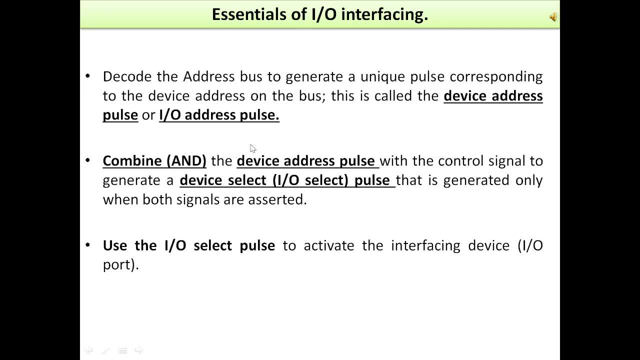 that is, this is the device address pulse with the control signal. to generate a device select pulse that is generated only when both the signals are asserted means we have to make sure that the microprocessor reaches the IO devices in a unique manner. that means, first of all, the instruction needs to be a IOMAP. 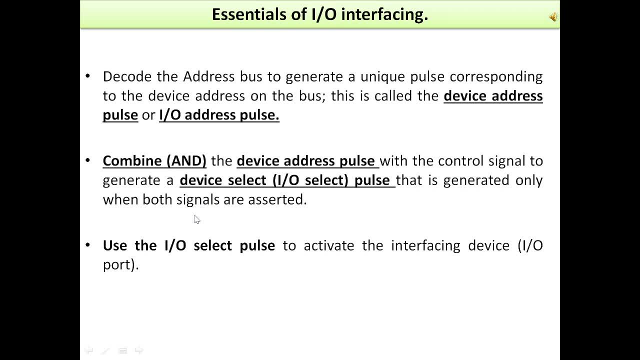 IO instruction. it has to be in or out. then the port address that are given should be decoded and along with the port address there should be a pulse coming from the IO read or IO write and combining only those two. only after that you should be able to generate a pulse. 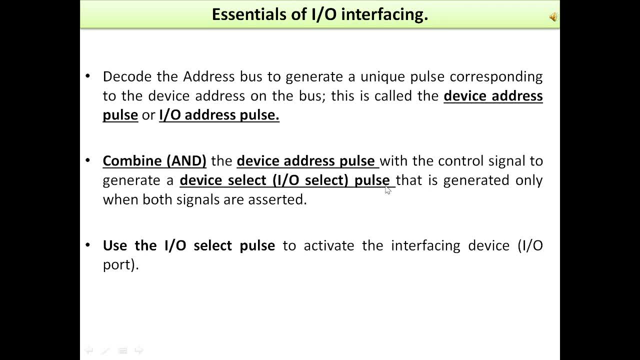 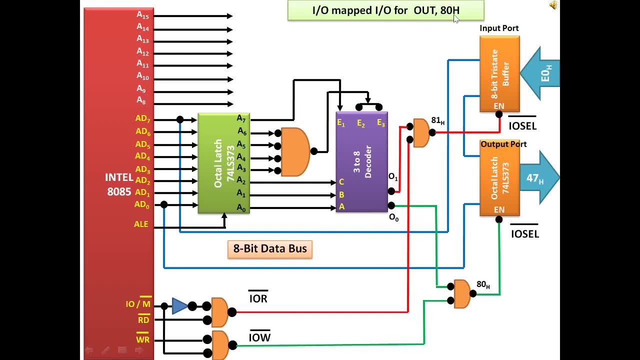 The input or the output port will be accessed. Let us now try and understand using this figure. now, let us assume that the input port addresses is 81 and the output port address is 80. Now, for instance, suppose the microprocessor is presently giving out an activator for a number of operators. In this caseit is assigned to Detect минут for dropdown, and under a parameter in my compile command I'll write input 2 for a input and output address for d1- Nt1, and a output port address for d2- Ntt, nt2 for the specific prop on the input carriers, whatever output interfaces are existing, and if the address's chipped, I will refer it to Node two, 18 and after a transformative next 했어요, the microprocessor is now� break the voluntary file". 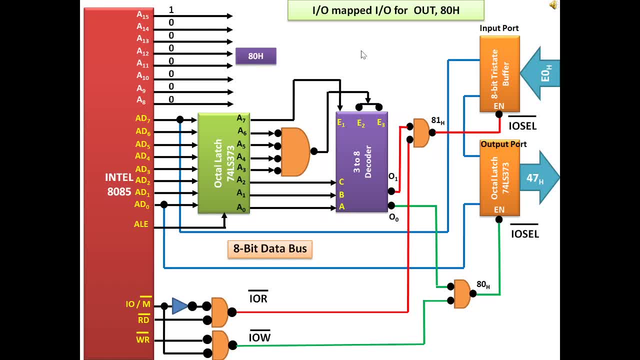 instruction which is out 80. that means presently the microprocessor is trying to communicate with the output, so the upper address bus information and the lower address bus information will be same as seen here. the same thing will be transferred to the output of the octal latch and the lower three bits are: 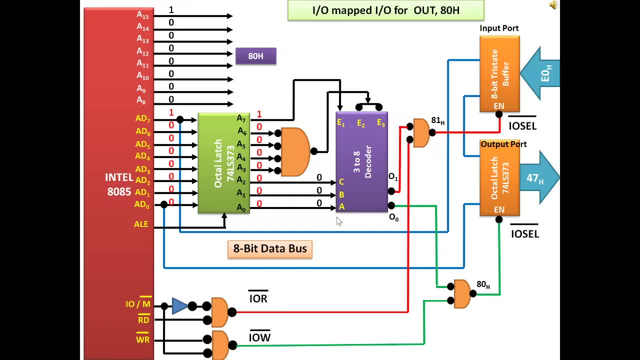 directly connected to the decoder and the one that is from a7 is directly connected to the active high enable of this latch. then a6, a5, a4 and a3 are decoded using a bubble NAND gate, where all are zero means the output will be zero, and it is connected to e2 and e3 where e2 and e3 are active. low type. 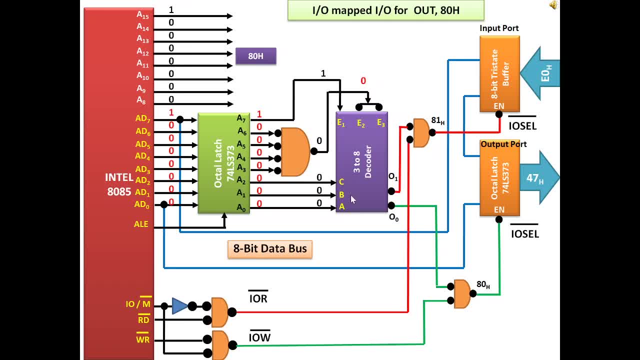 interface enable. so a7 to a3. all this signal ensures that this particular decoder is active. now, when it is 0, 0, 0 here, we will get the o 0 output high. so we have generated a device select pulse. take it, it is the device address pulse now use. 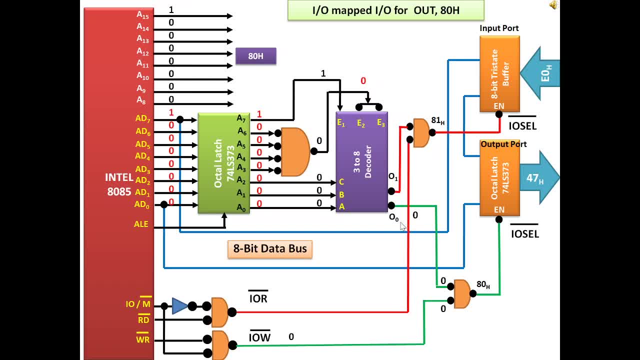 it is an output port we will be using, are you right? which is 0 right now, because the instruction is out. so this 0 and this 0 will create a low pulse at the output of this and hence this will get activated. but what about the other? 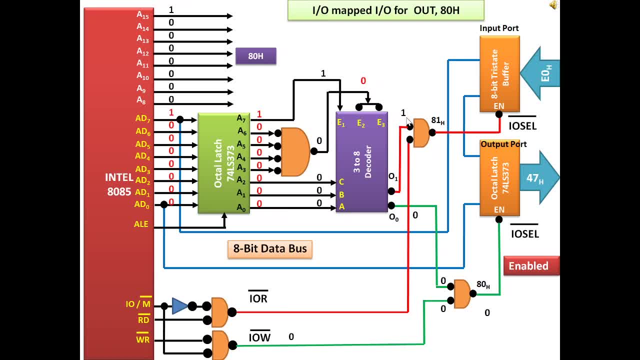 port, the other port, you can see, since it is 0, 0, 0 here, this o 1 will be high, and when the microprocessor is in the write mode it cannot be in the read mode. so this is high. so one and one will create a one at the output, and hence the input port is presently disabled. 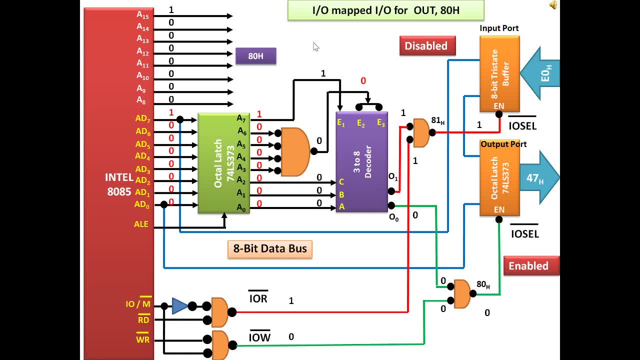 so what we can see is, when the microprocessor is generating out 80, it is uniquely identifying the output port and the content which is presently available in the accumulator, which was 47, will be available at the output of this. similarly, let us try to understand if the microprocessor is trying to get a 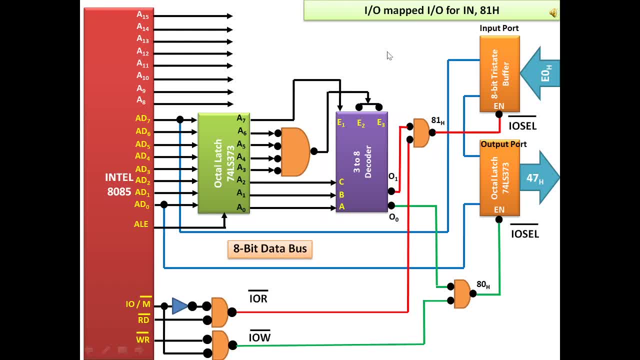 information from the outside world into it using the import or the in instructions. now let's see. the microprocessor is presently generated 81 hex. that means it is presently trying to execute in 81 instruction. so similarly the upper address bus and the lower address bus will have the same information. now the latch. 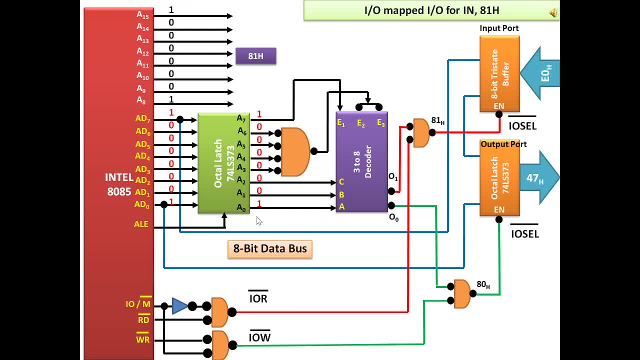 because of ali, the same information will be available outside the latch and since the lower three are 0, 0, 1, it will actually enable the output o1, but for that we need to enable the entire decoder to do that. we have a 1 from a7 and we have a 0 from the purple than gate, so this signal ensures 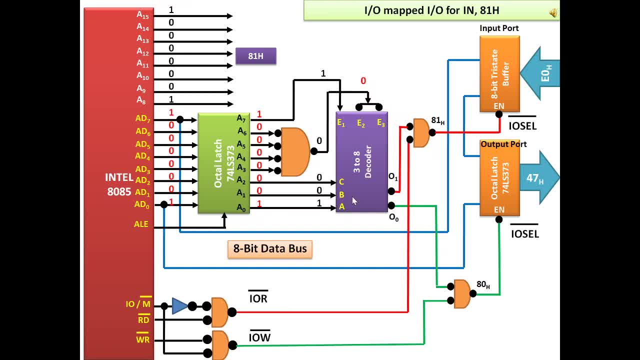 that the decoder is active and this ensures that the o1 is active. so what we can see is this is our seesan from the input. so this is the part says read mode. this bit is just here, and since this is zero, zero one, this will become deactivated and hence it is these disabled the output port. 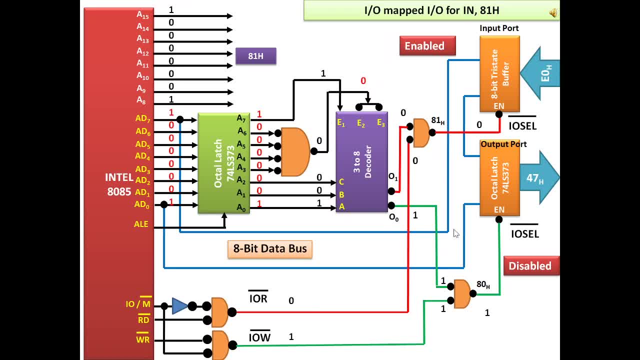 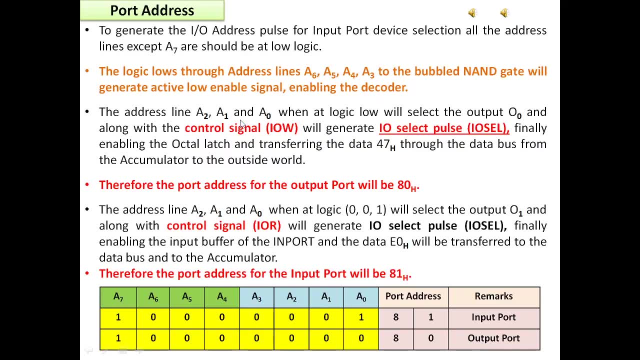 the port is now will be transferred through the data bus into the accumulator. So far we have seen that to generate IO address pulse for input port device selection, all the address lines except A7 are at ground low. Now this is because A7 is directly connected. 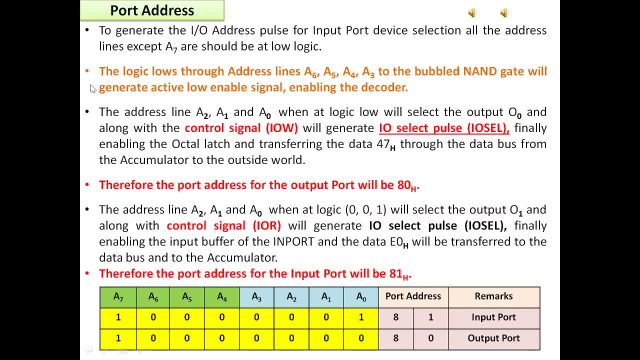 to the active high enable input of the decoder. The logic low through address lines A6, A5, A4, A3 are directly connected to the bubble NAND gate. This will generate an active low enable signal which will enable the decoder. Now A2, A1 and A0 are directly 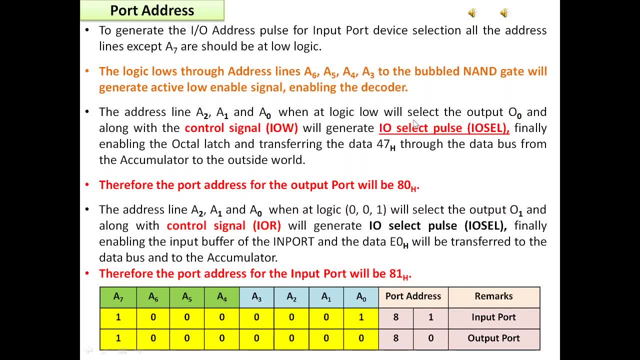 connected to the email input picture of the decoder as well. input of the 3 line to 8 line decoder. Now the output of the decoder O0 will get selected when A2, A1 and A0 are low, Along with the control signal. we can select either the output. 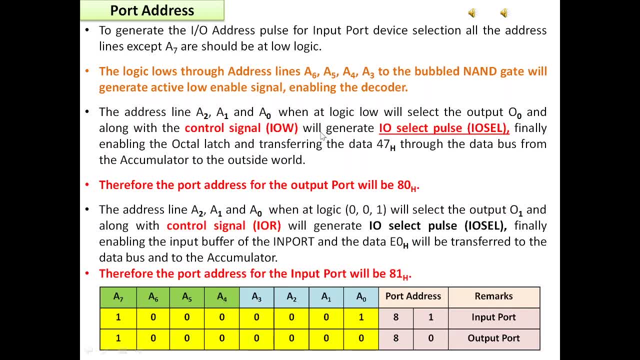 port or the input port? Okay, so if we are talking about the output port, then the address lines A2, A1 and A0 are, at logic, low will select the output O0 and, along with the control signal IOW, that is, IO right, will generate a IO select pulse. Finally, enabling the octal, 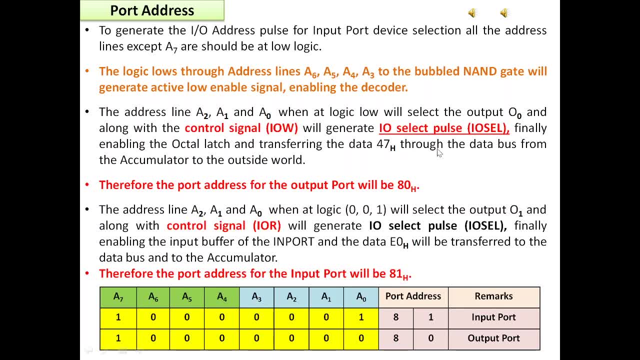 latch And transferring the data 47 through the data bus from the accumulator to the outside world. Therefore, the port address for the output port will be 8: 0.. Similarly, the address lines A2,, A1,, A0, when at logic 0,, 0,, 1, will select the output O1 and along with the control.